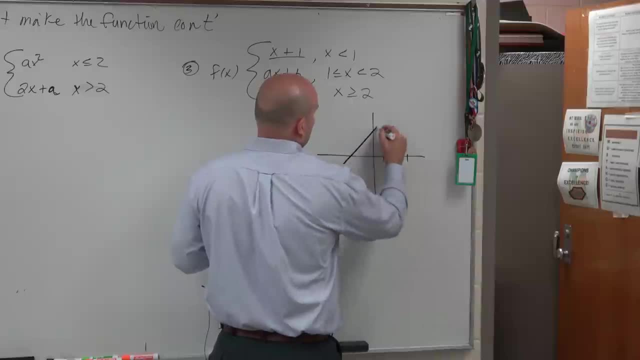 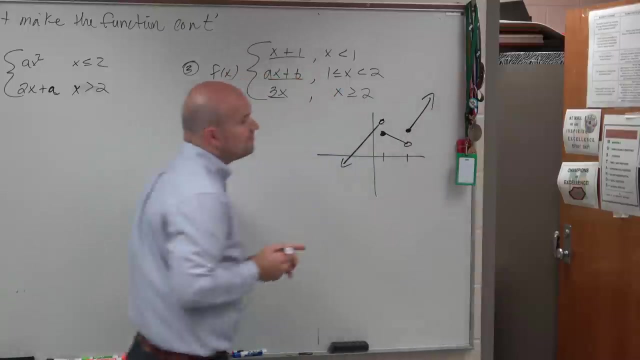 So I'm just going to say here, a graph looks like this, Then a graph looks like that, That's open, And that's open, And then a graph looks like this. So basically, what we're trying to do is we're trying to connect these three graphs. 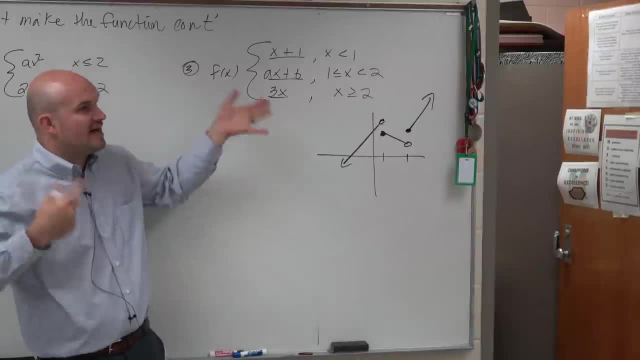 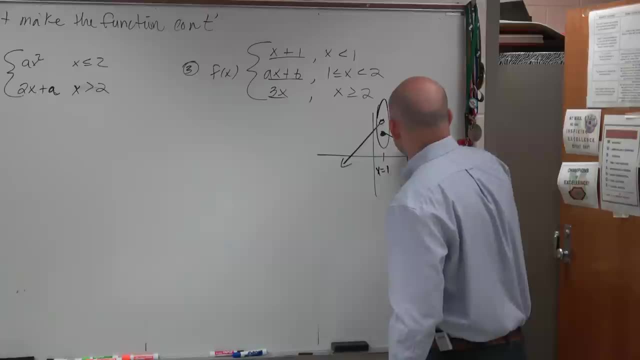 so the graph is continuous. That's what we're trying to do. We're trying to find the values that are going to make these connections. So, basically, there's two values that we want to have connected: at x equals 1 and at x equals 2.. 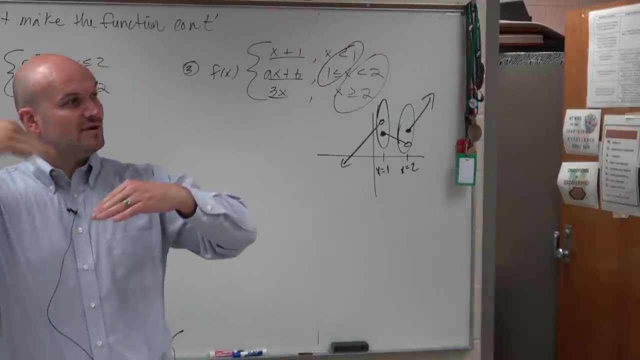 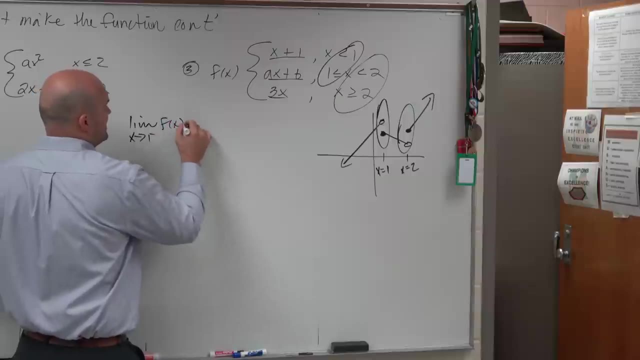 You guys see that. So for them to be connected, they know that the left and the right-hand limits need to be the same. So we'd say that the limit as x approaches 1 from the left of f of x has to equal the limit as x approaches. 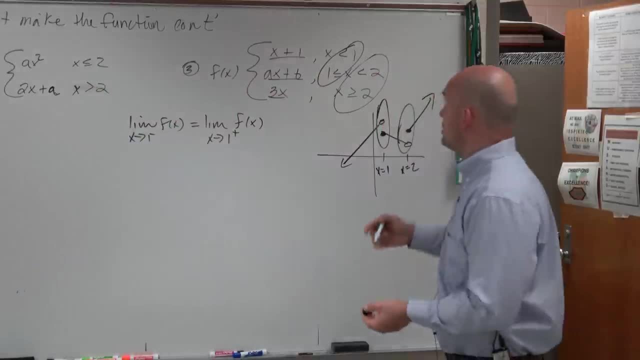 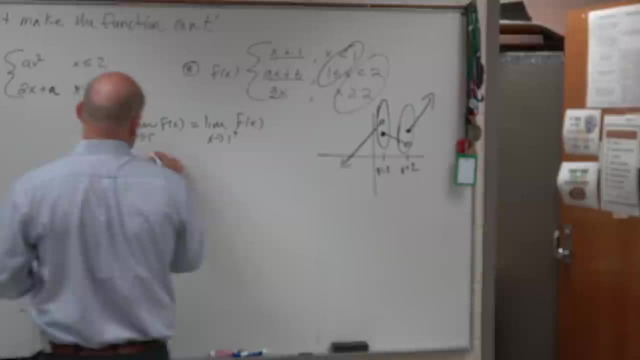 1 from the right of f, of x. So we basically want to make sure these are the same from the left and right hand, because right now they're not the same right. So to make them the same, we're just going to do: 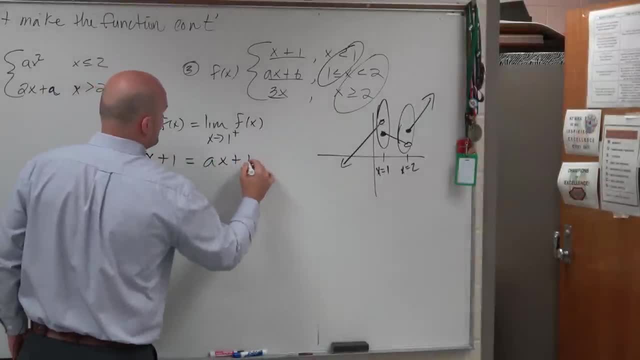 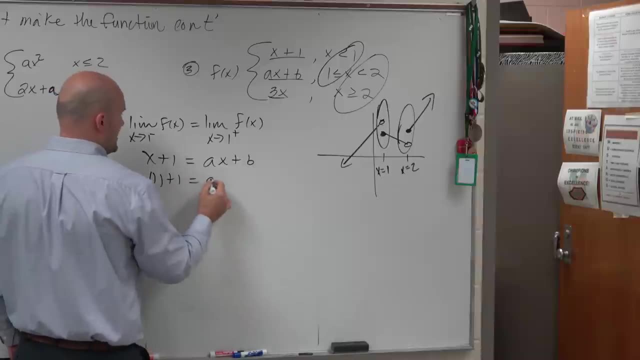 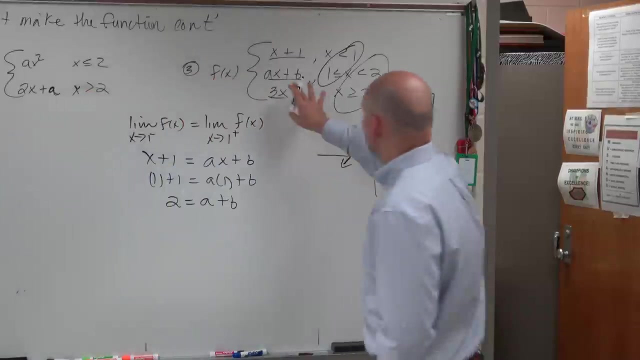 so x plus 1 has to equal ax plus b. Now you evaluate in the limit. So therefore you're going to plug in: 1 plus 1 equals a times 1 plus b. So your first equation is: 2 equals a plus b. 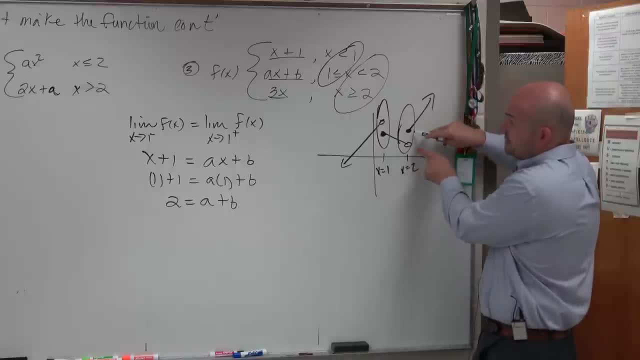 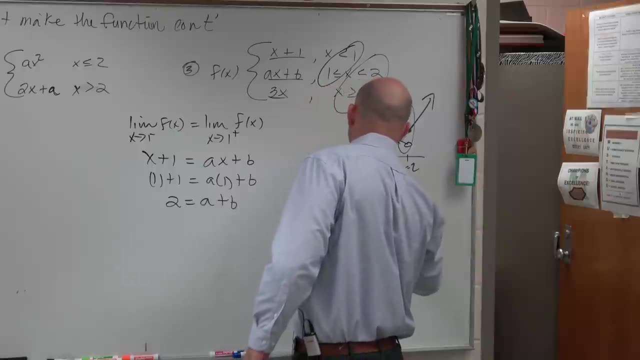 For the next thing, we want to make sure the left and right-hand limit at 2 is going to be the same. So again, I'll just write the limit as x approaches 2 from the left of f of x equals the limit as x approaches 2. 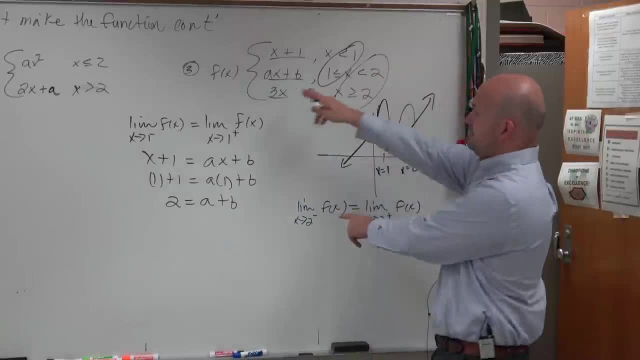 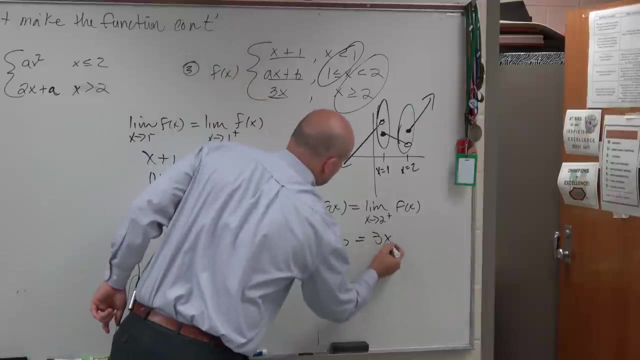 from the right of f of x. So the left-hand limit is ax plus b And the right-hand limit is ax plus b, And the right-hand limit is ax plus b And the right-hand limit is going to be what represents 3x. 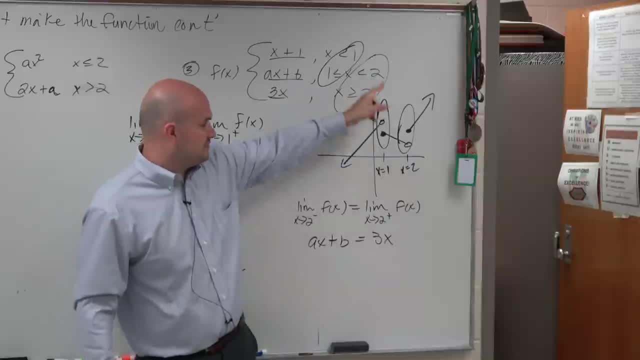 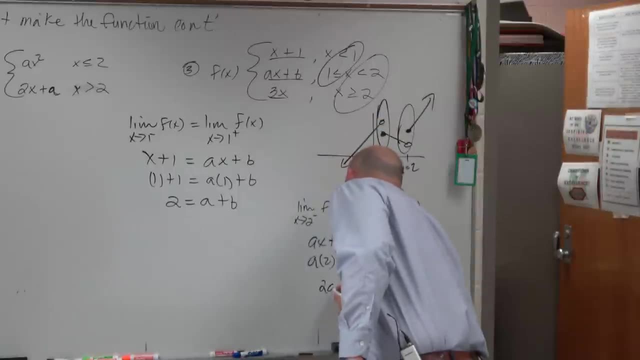 Then I plug in my new value that I'm trying to make them connect at, which is 2.. So it's going to be: a times 2 plus b equals 3 times 2, which is 2a plus b equals 6.. 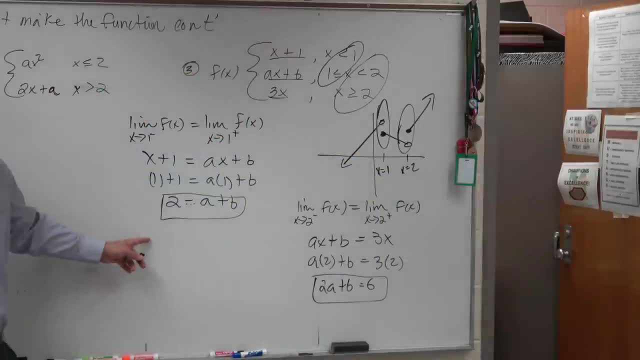 So there's one equation, There's my other equation. Now that I have these two equations, I can just use a system of equations to solve: a plus b equals 2. And 2a plus b equals 6.. So I just rewrote them. 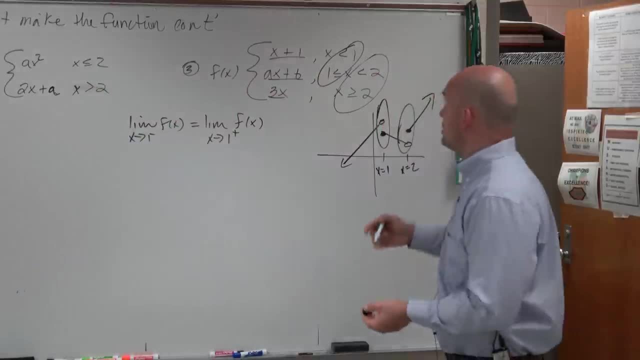 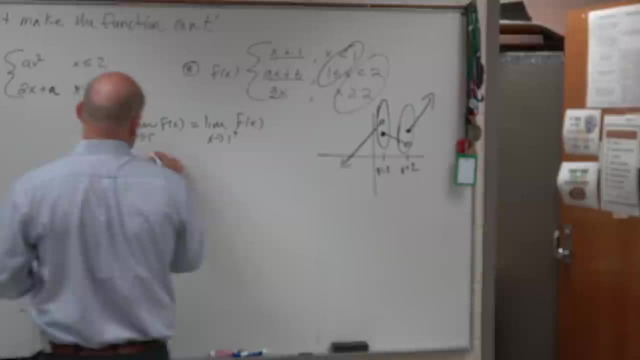 1 from the right of f, of x. So we basically want to make sure these are the same from the left and right hand, because right now they're not the same right. So to make them the same, we're just going to do: 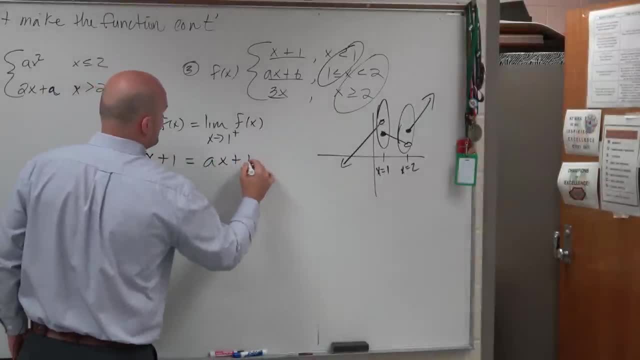 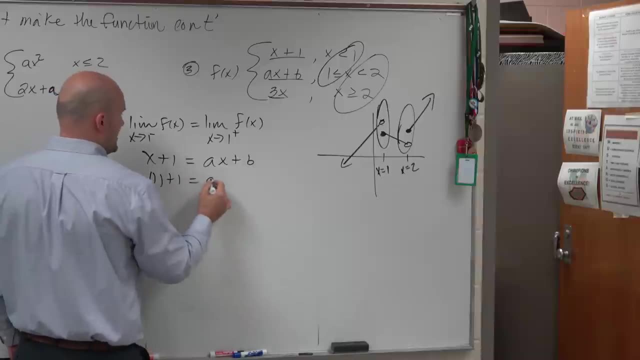 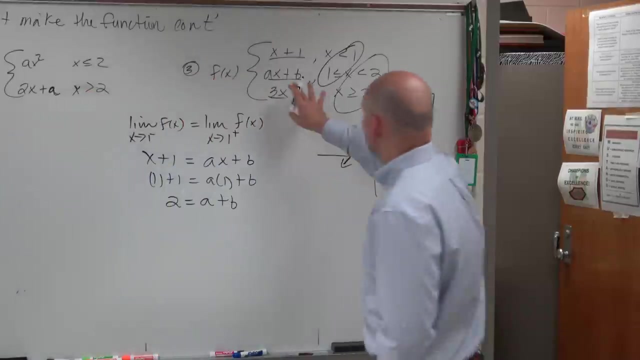 so x plus 1 has to equal ax plus b. Now you evaluate in the limit. So therefore you're going to plug in: 1 plus 1 equals a times 1 plus b. So your first equation is: 2 equals a plus b. 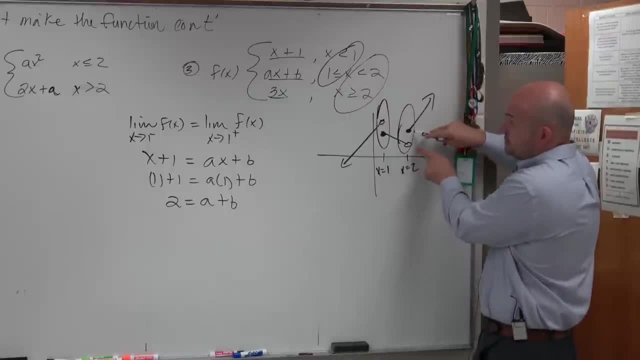 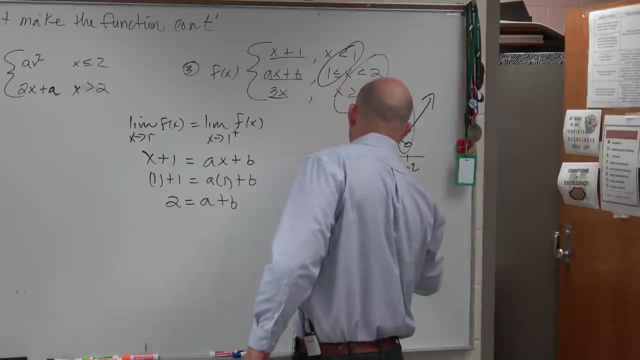 For the next thing, we want to make sure the left and right-hand limit at 2 is going to be the same. So again, I'll just write the limit as x approaches 2 from the left of f of x equals the limit as x approaches 2. 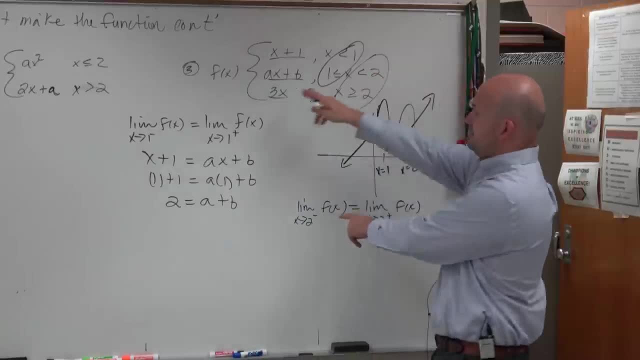 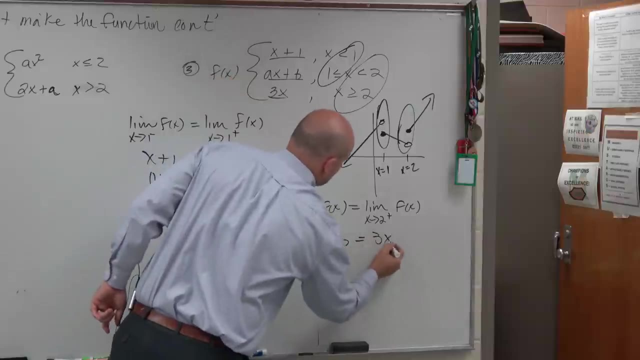 from the right of f of x. So the left-hand limit is ax plus b And the right-hand limit is going to be what represents 3x. Then I plug in my new value that I'm trying to make them connect at, which is 2.. 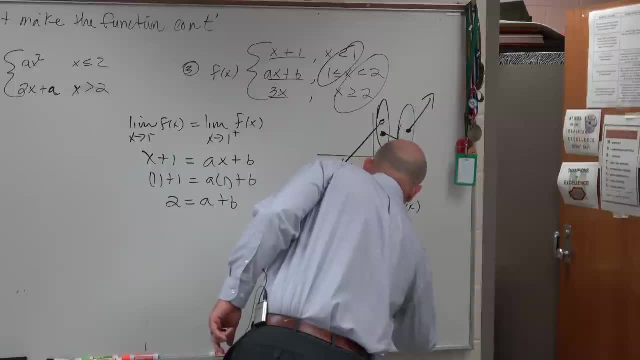 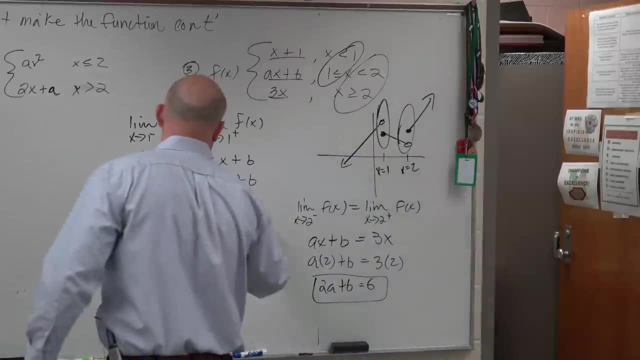 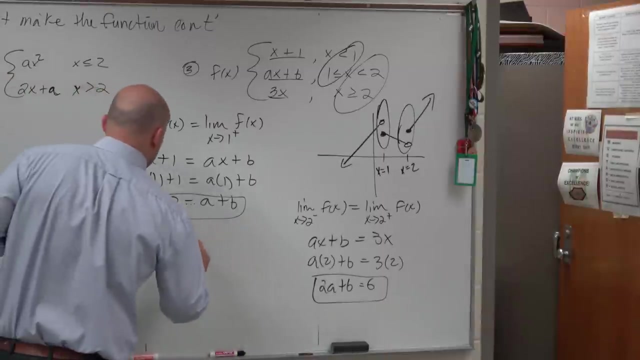 So it's going to be: a times 2 plus b equals 3 times 2, which is 2a plus b equals 6.. So there's one equation. There's my other equation. Now that I have these two equations, I can just use a system of equations to solve. 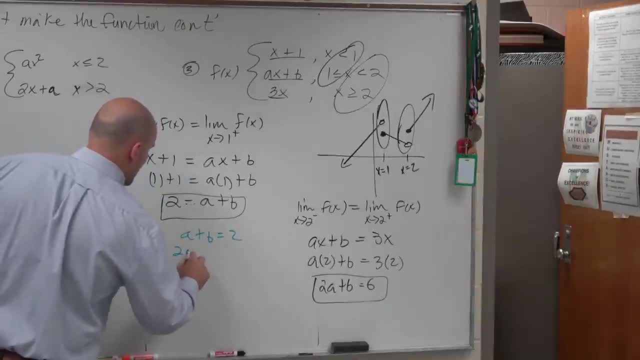 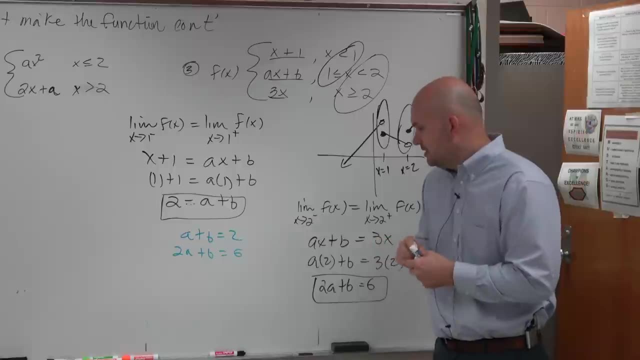 a plus b equals 2.. And I plug in my new value: And 2a plus b equals 6.. So I just rewrote them. You don't need to rewrite them, but that's the way I like to do it. 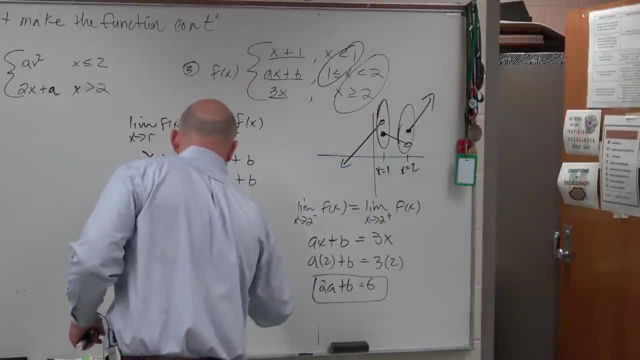 And then I'm going to use elimination. So what I'm going to do is I'm going to subtract the two. So by subtracting the two equations from one another, I get negative a minus 0b equals negative 4.. So it's negative a equals negative 4.. 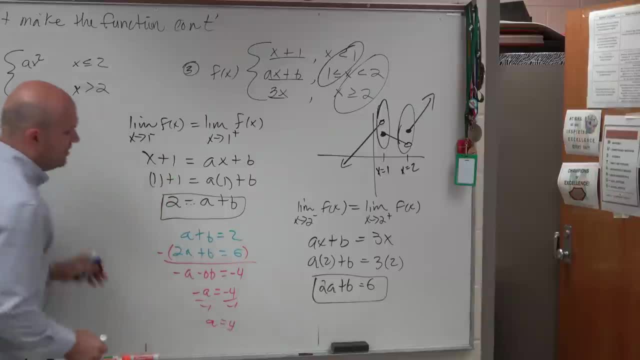 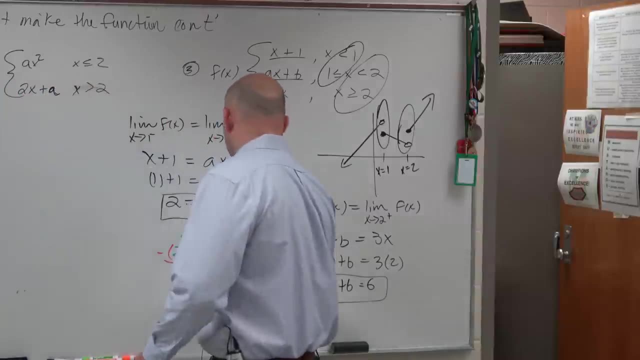 Divide by negative: 1.. Divide by negative 1.. a equals 4.. And then, now that I know what a equals 4 is, to find out b, I just plug it into one of these other two equations. So let's plug it in here. 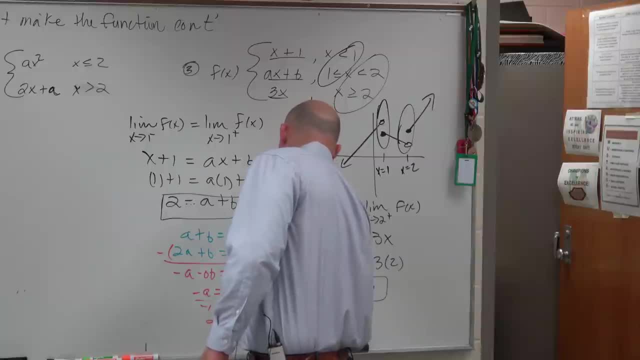 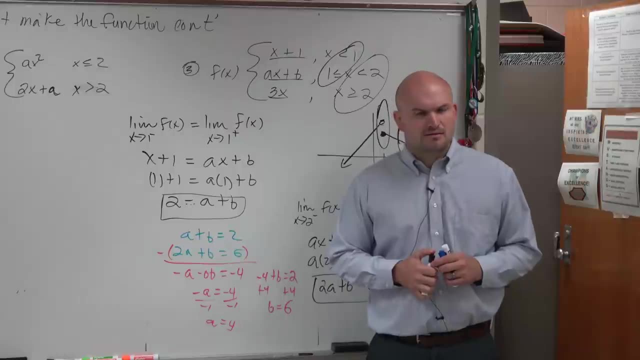 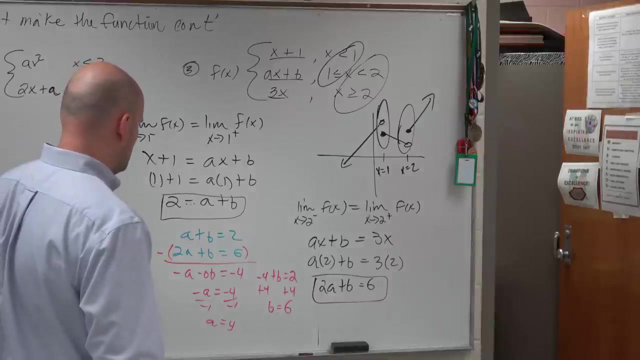 Negative: 4 plus b equals 2.. Add 4.. Add 4. b is equal to 6.. Was that the answer? negative 4 and 6?? No, What happened? It's negative 2.. b is negative 2..